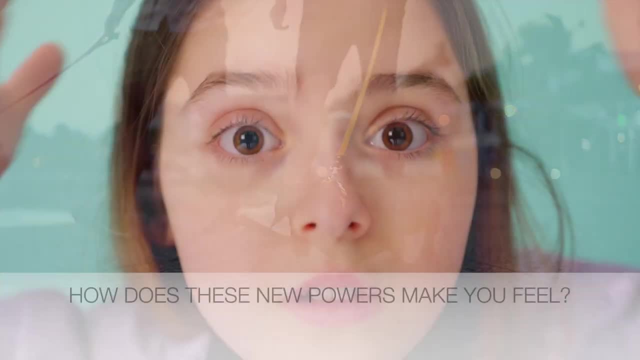 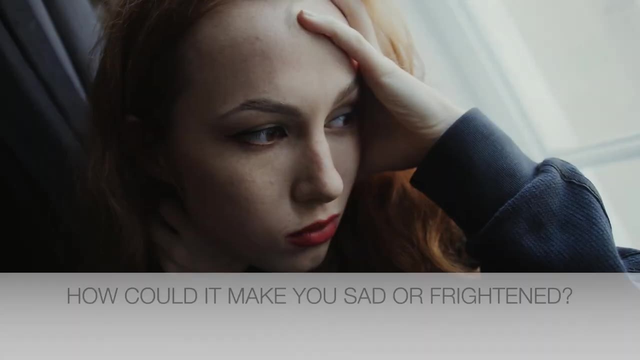 If you have a pet, what would they say to you? To add more interesting things to your character's interactions, think about how they might feel. Words like bewildered, ecstatic and apprehensive can bring your story to life. Now let's tackle. 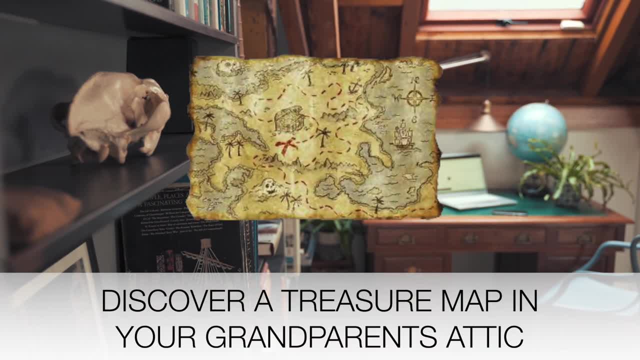 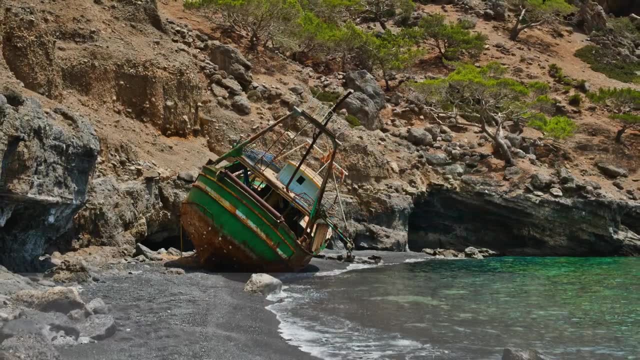 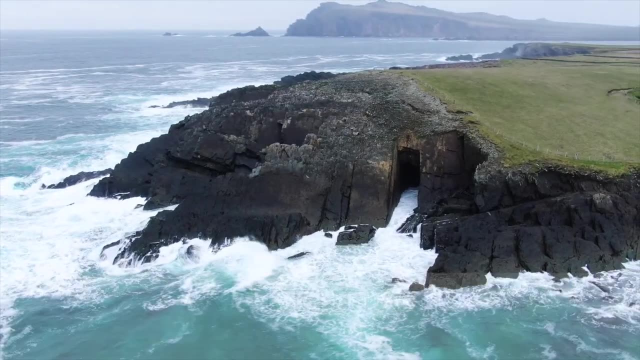 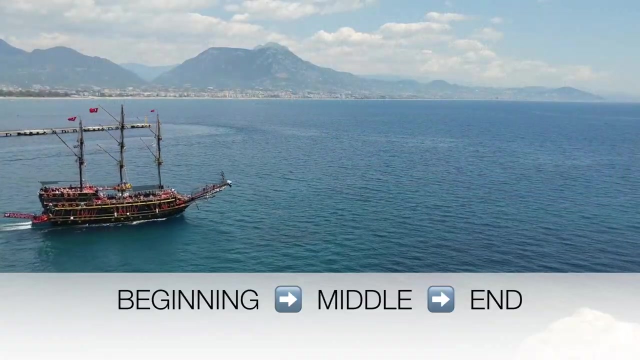 prompt non-stop Number two: you discover a hidden treasure map in your grandparents' attic. As you explore this prompt, consider the setting and the journey your characters will undertake. Will they face challenges, Encounter danger Or uncover unexpected surprises? To keep your readers engaged, create a clear beginning, middle and end. 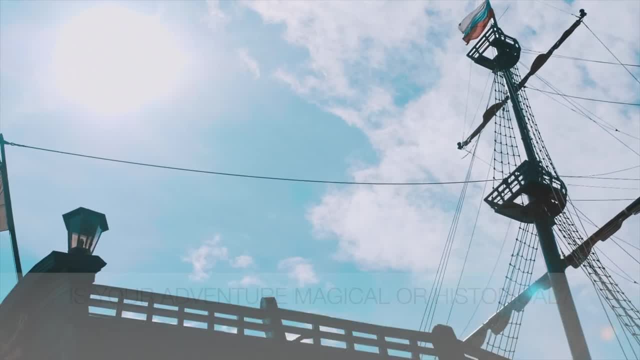 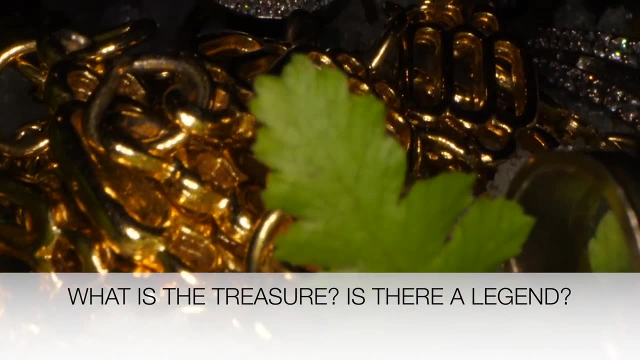 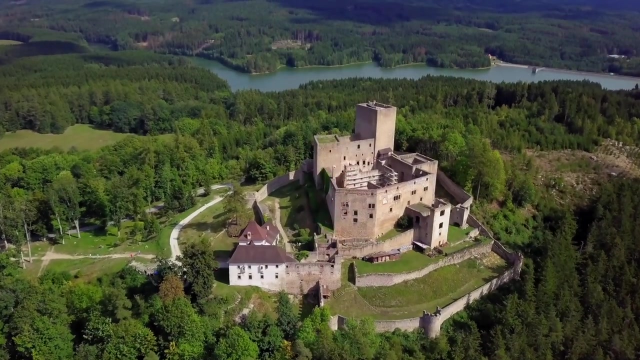 Use descriptive language with lots of adjectives to paint a vivid picture. picture of the map, the characters and the places they'll visit. Think about the treasure itself. Is there a legend attached to the treasure, or maybe a curse? Will your adventure be based on history, with kings and pirates, or will 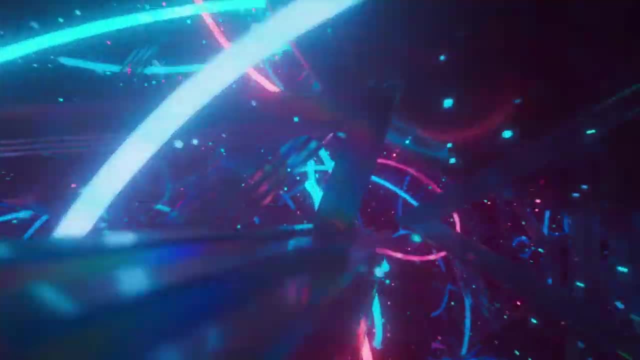 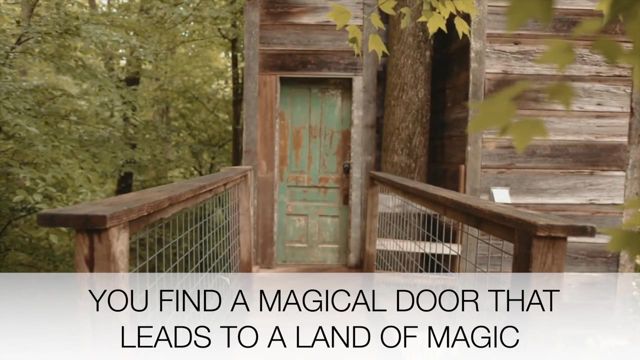 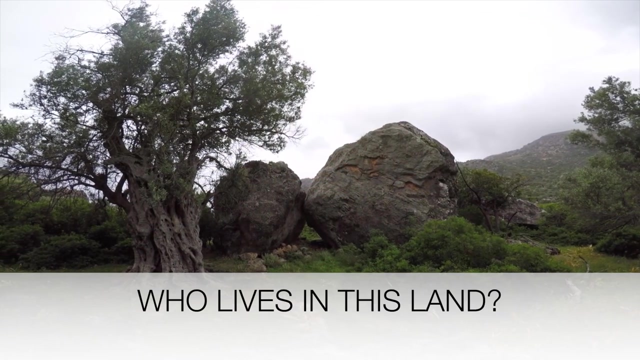 it be based on magic, with witches and wizards. Prompt number three invites us to explore the world of fantasy. You find a magical door that leads to a land of magic. Think about the magical creatures you'll encounter and the landscapes you'll explore. Think about the adventures that await beyond the door. 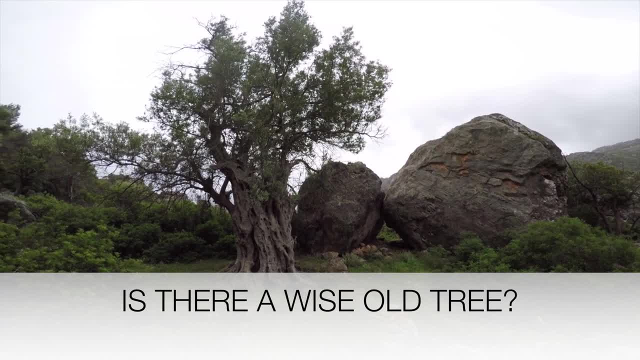 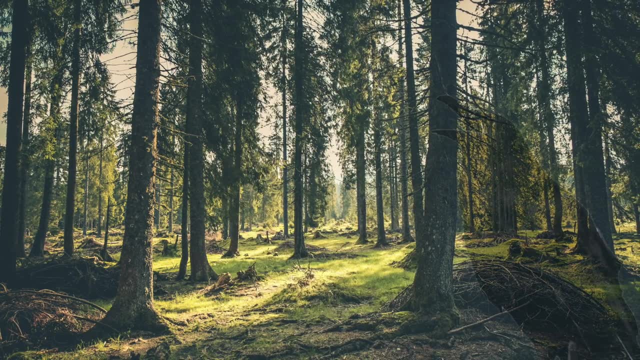 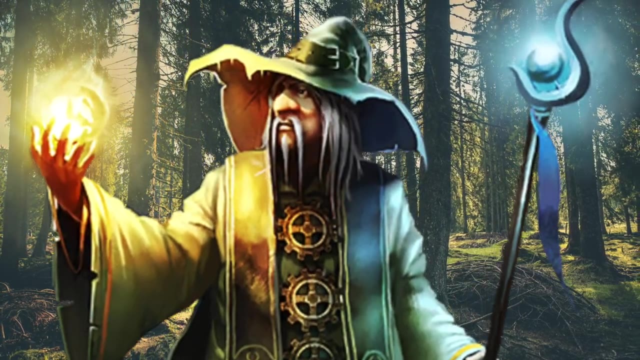 Use sensory details to immerse your readers in this enchanting world. It's important to give your characters distinct voices and personalities. How would a chatty crow sound? Or how about a wise old wizard? Dialogue can reveal a lot about your characters. 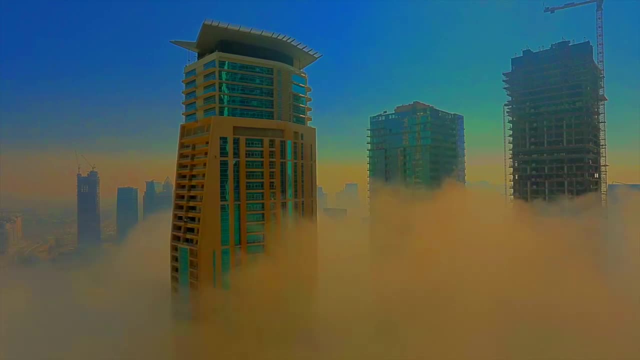 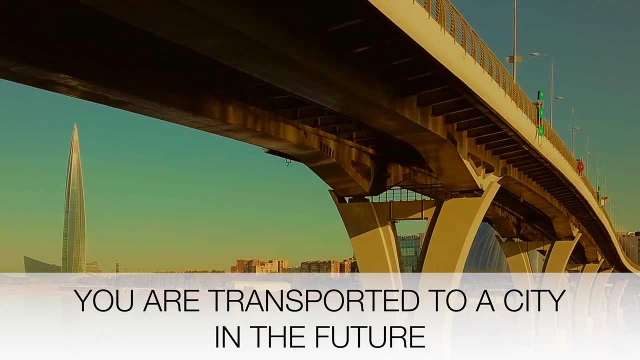 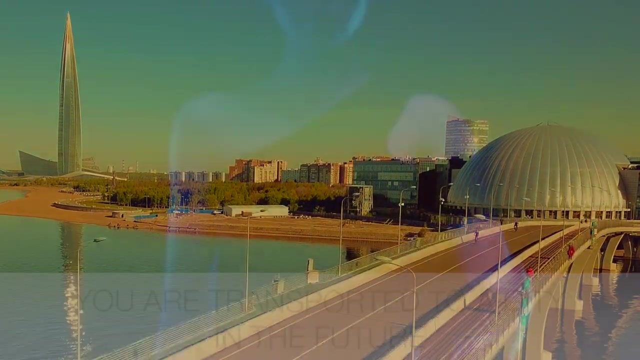 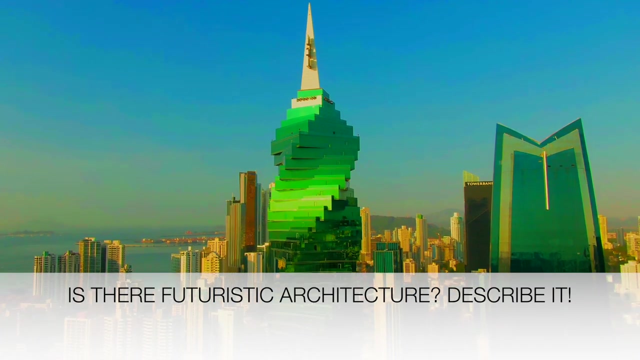 traits. Our final prompt takes us to the bustling streets of a city. You are transported to a city in the future, a place full of unbelievable technology and where humans and robots coexist. Imagine the different types of advanced technology, the futuristic architecture and the cultural changes. How does this? 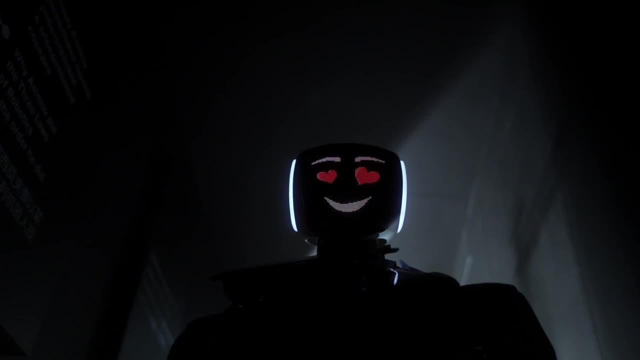 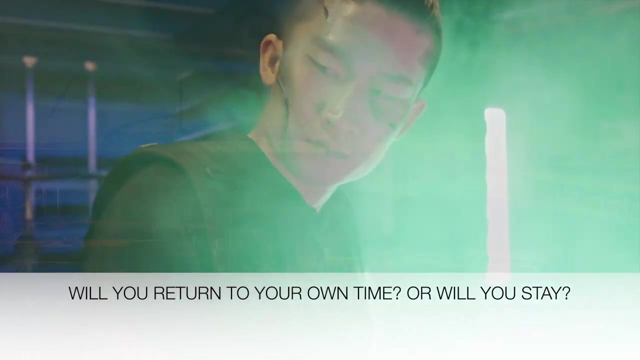 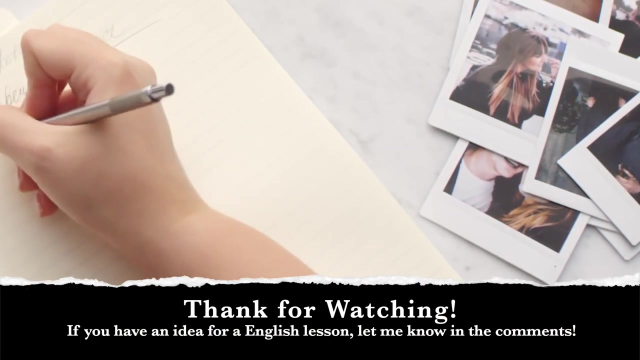 new technology affect day-to-day life. What are the challenges that people in this era of history face? And a big question: will you return to your own time or will you stay in the future? And there you have it: four captivating writing prompts to fuel your creativity and improve your writing skills.